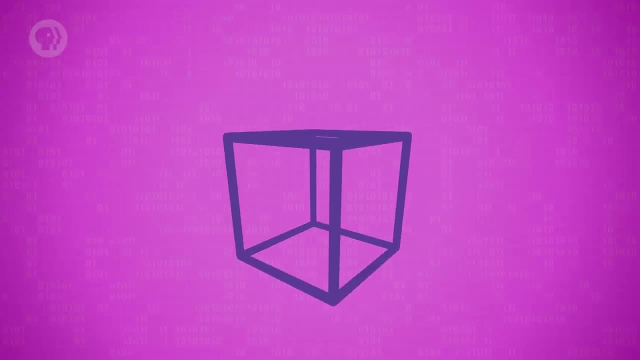 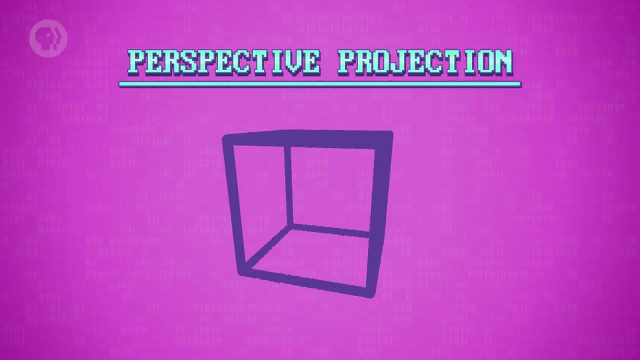 projection In the real 3D world, though parallel lines converge as they get further from the viewer, like a road going to the horizon. This type of 3D projection is called perspective projection. It's the same process just with different math. 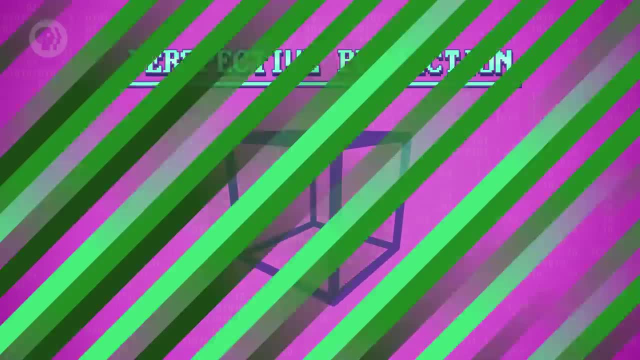 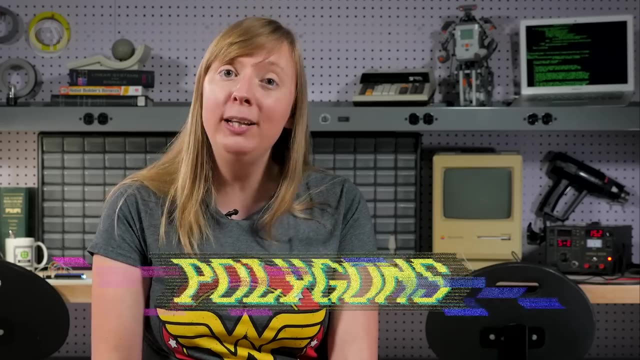 Sometimes you want perspective and sometimes you don't. The choice is up to the developer. Simple shapes like cubes are easily defined by straight lines, But for more complex shapes, triangles are better- what are called polygons in 3D graphics. Look at this beautiful teapot made out of polygons. A collection of polygons like this. 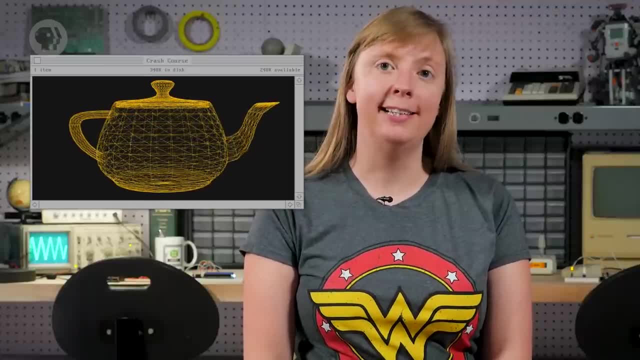 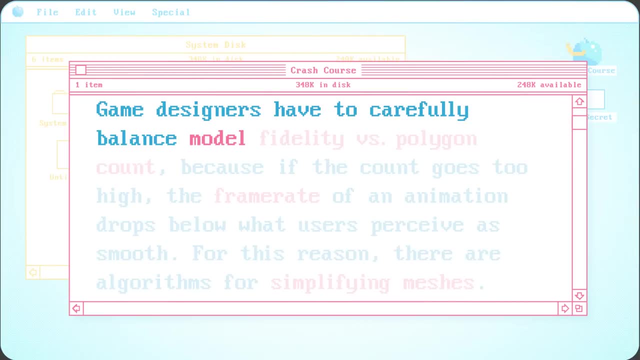 is a mesh. The denser the mesh, the smoother the curves and the finer the details. But that also increases the polygon count, which means more work for the computer. Game designers have to carefully balance model fidelity versus polygon count because they don't know how to do it. 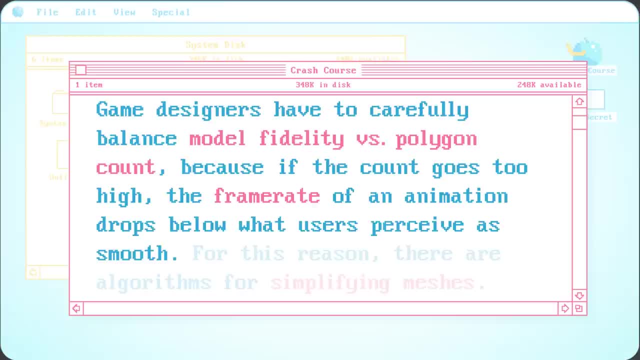 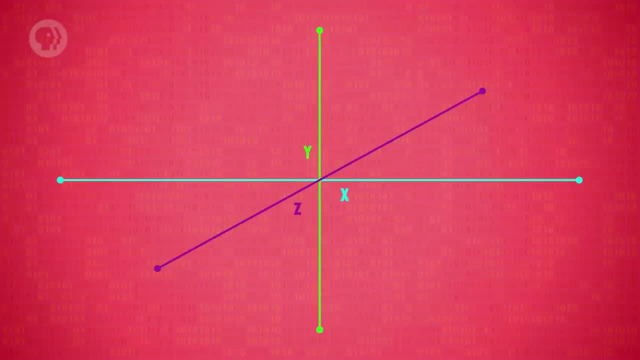 If the count goes too high, the frame rate of an animation drops below what users perceive as smooth. For this reason, there are algorithms for simplifying meshes. The reason triangles are used and not squares or polygons or some other more complex shape is simplicity. Three points in space can ambiguously define a plane If you give me three points. 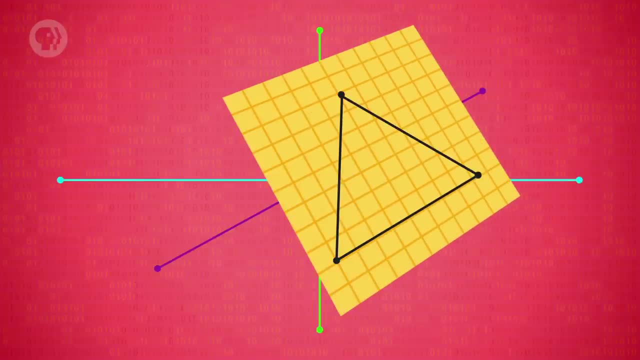 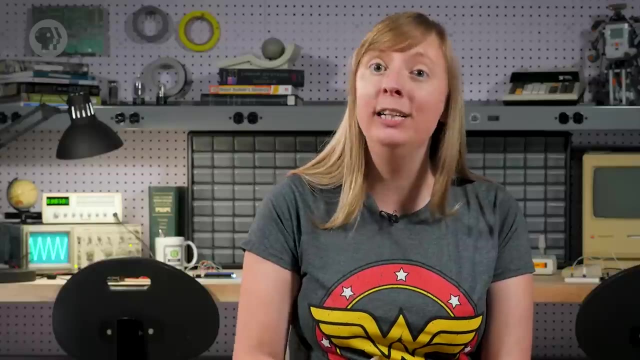 in a 3D space, I can draw a plane through it. There is only one single answer. This isn't guaranteed to be true for shapes with four or more points. Also, two points aren't enough to define a plane, only a line. 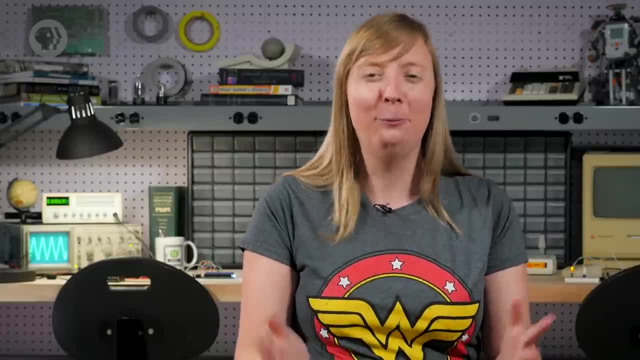 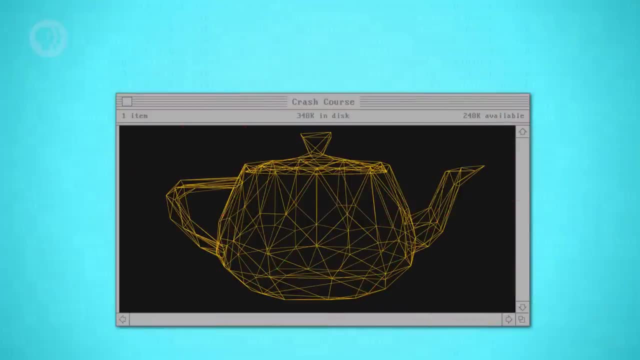 So three is the perfect and minimal number. Triangles for the win. Wireframe rendering is cool and all sort of retro, but of course 3D graphics can also be filled. The classic algorithm for doing this is called scanline rendering, first developed in 1967. 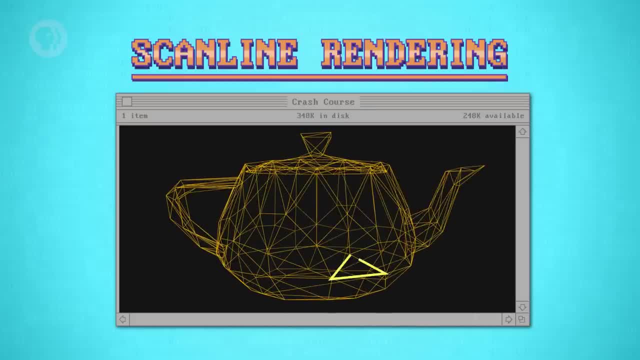 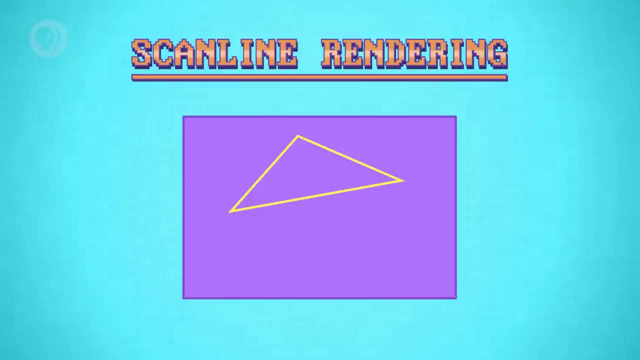 at the University of Utah. For a simple example, let's consider just one polygon. Our job here is to figure out how this polygon translates to filled pixels on a computer screen. So let's first overlay a grid of pixels to fill. The scanline algorithm starts by reading the three points that make up the 3D space: The. 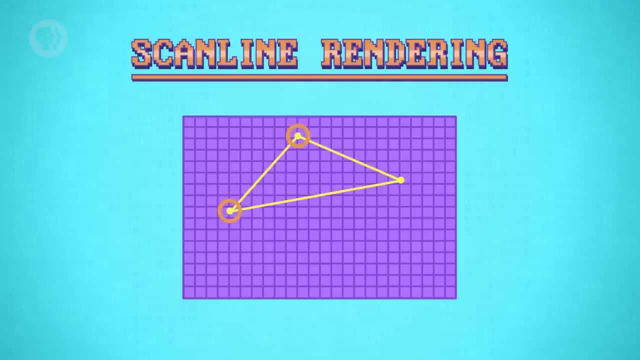 3D space is the number of pixels that make up the polygon, and finding the lowest and highest y values. It will only consider rows between these two points. Then the algorithm works down one row at a time. In each row it calculates where a line 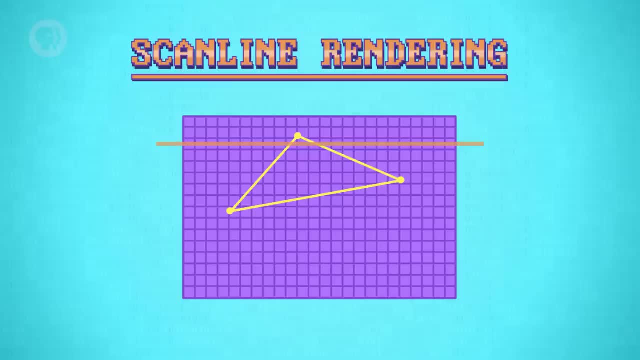 running through the center of a row intersects with the side of the polygon, Because polygons are triangles. if you intersect one line, you have to intersect with another. It's guaranteed. The job of the scanline algorithm is to fill in the pixels between the two intersections. 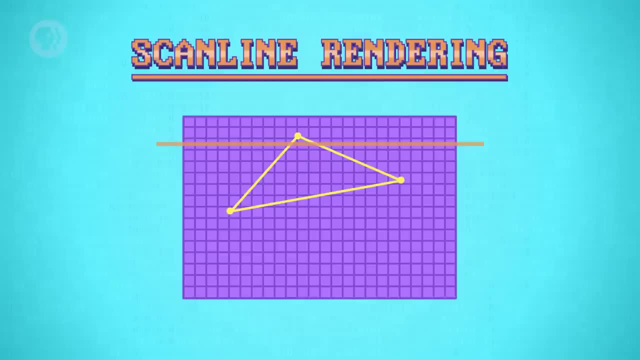 Let's see how this works. On the first row we look at, we intersect here and here. The algorithm then colors in all the pixels between those two intersections And this just continues row by row, which is why it's called scan line rendering. 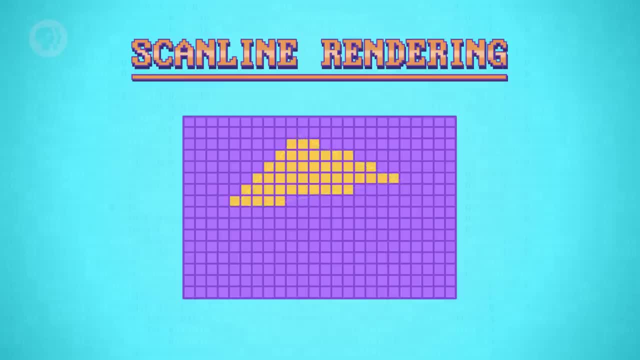 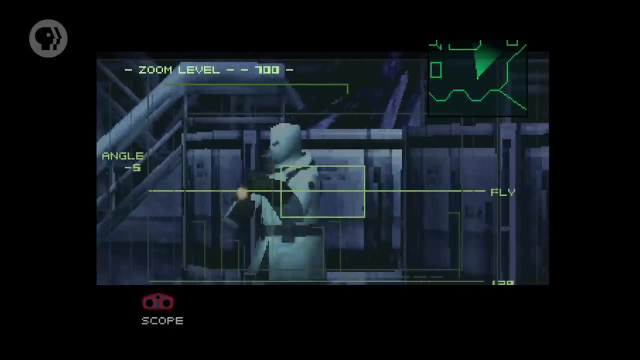 When we hit the bottom of the polygon, we're done. The rate at which a computer fills in polygons is called the fill rate. Admittedly, this is a pretty ugly filled polygon. It has what are known as jaggies, those rough. 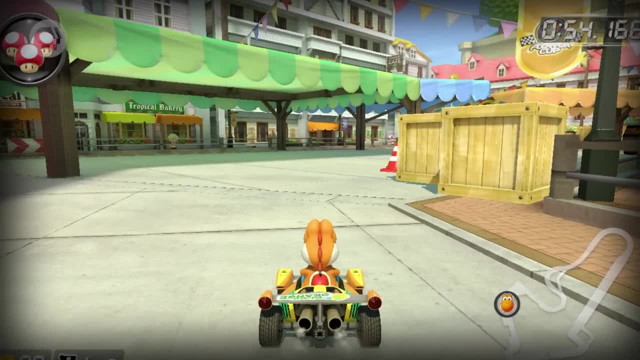 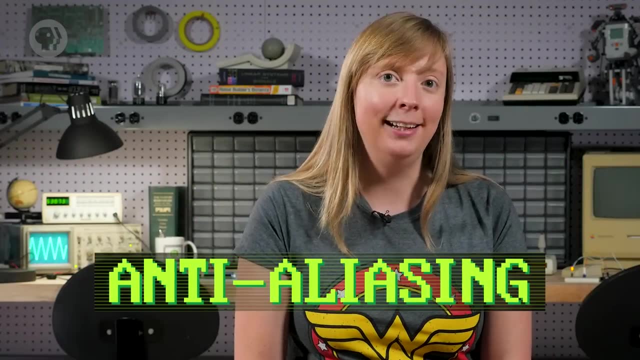 edges. This effect is less pronounced when using smaller pixels, but nonetheless you see these in games all the time, especially on lower powered platforms. One method to soften this effect is anti-aliasing. Instead of filling pixels in a polygon with the same color, we can adjust the color based. 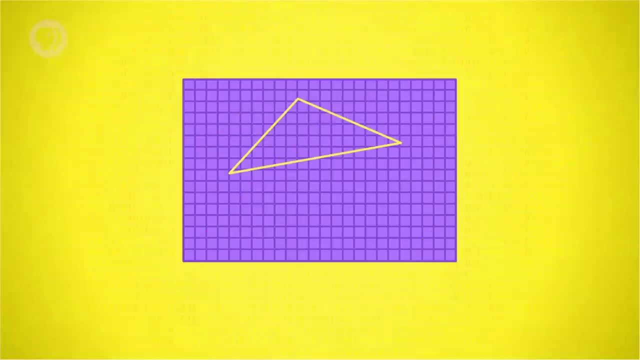 on how much the polygon cuts through each pixel. If a pixel is entirely inside of a polygon, it gets fully colored, But if the polygon only grazes a pixel, it'll get a lighter shade. This feathering of the edges is much more pleasant to the eyes. Anti-aliasing is used all over the place, including in 2D graphics like fonts and icons. If you lean in real close to your monitor, closer, closer you'll see. all the fonts in your browser are anti-aliased, So smooth. 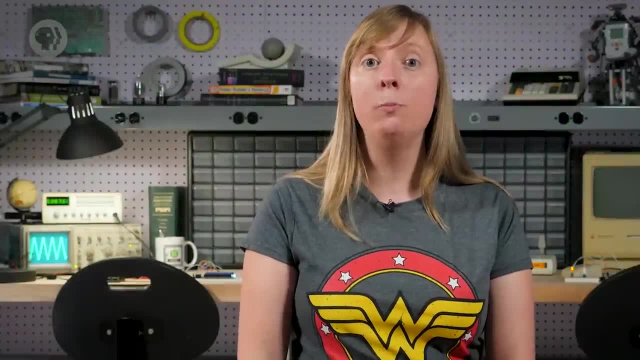 I'm going to show you how to do that in just a second. In a 3D scene there are polygons that are part objects in the back, near the front and just about everywhere. Only some are visible because some objects are hidden behind other. 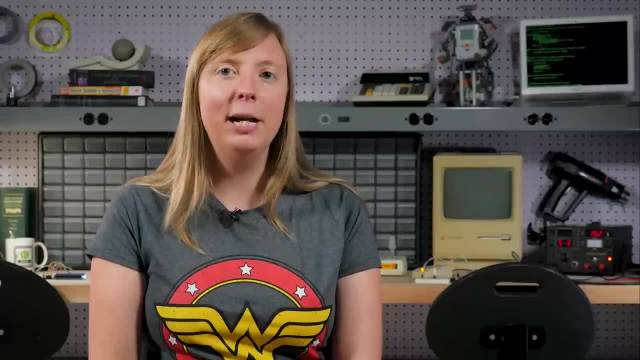 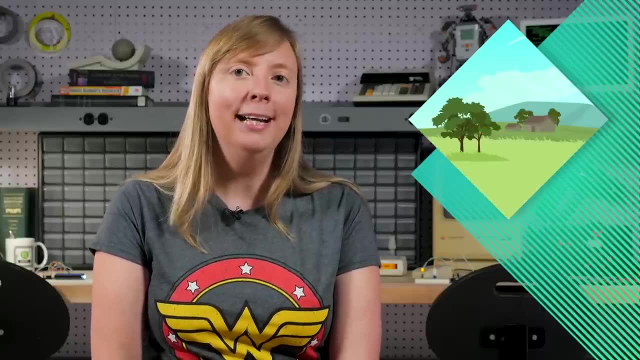 objects in the scene, What's called occlusion. The most straightforward way to handle this is to use a saw algorithm and arrange all the polygons in the scene from farthest to nearest, then render them in that order. This is called the painter's algorithm, because painters also have to start with the background. 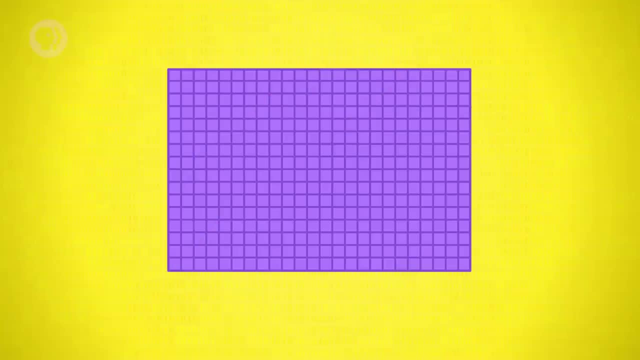 and then increasingly work up to foreground elements. Consider this example scene with three overlapping polygons. To make things easier to follow, we're going to colour the polygons differently. Also for simplicity, we'll assume these polygons are all parallel to the screen, But in a real 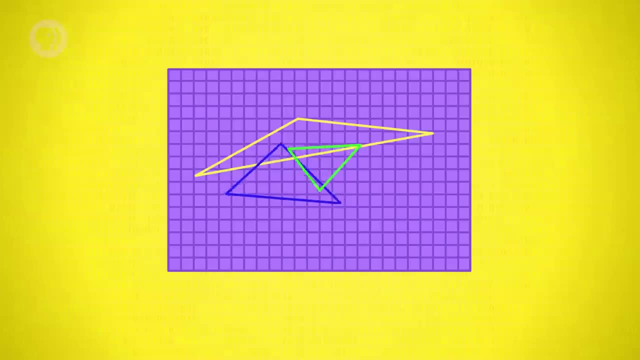 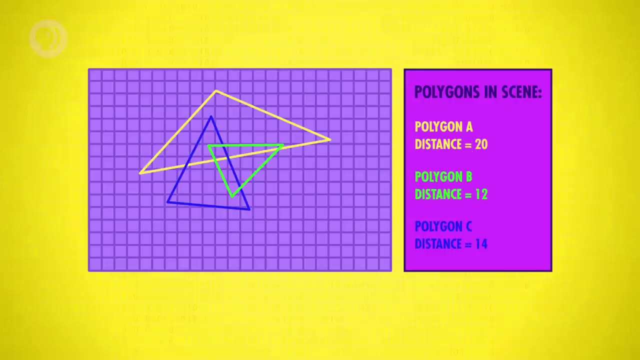 program like a game. the polygons can be tilted in 3D space. Our three polygons, A, B and C, are at distance 20,, 12, and 14.. The first thing the painter's algorithm does is sort all the polygons from farthest. 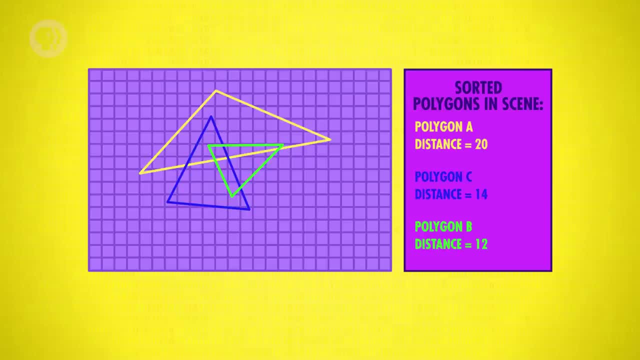 to nearest. Now that they're in order, we can use scanline rendering to fill each polygon one at a time. We start with polygon A, the furthest one away, Then we repeat the process For the next farthest polygon, in this case C, And then we repeat this again for polygon. 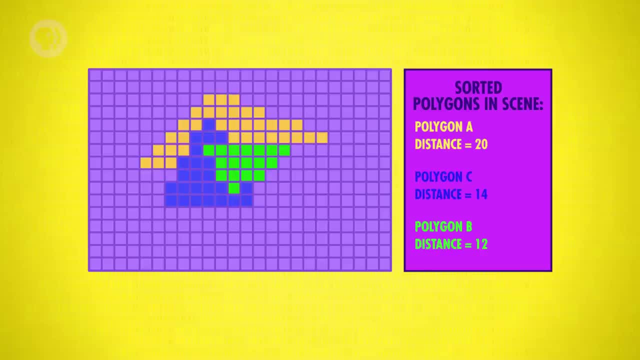 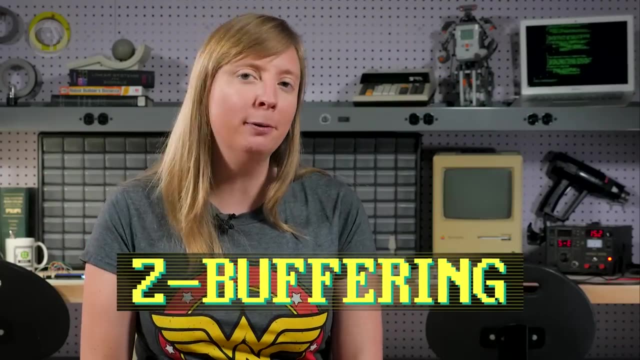 B. Now we're all done and you can see the ordering is correct. The polygons that are closer are in front. An alternative method for handling occlusion is called Z-buffering. It achieves the same output as before, but with a different algorithm. 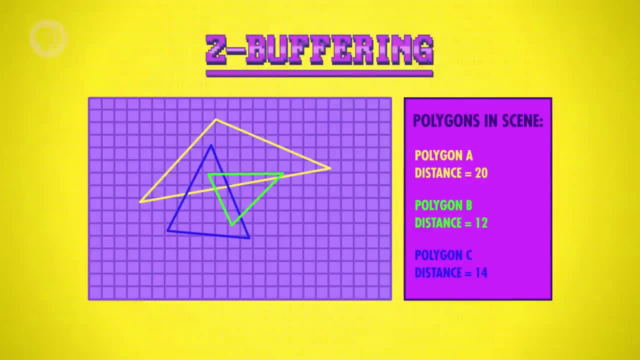 Let's go back to our previous example, before it was sorted. That's because this algorithm doesn't need to sort any polygons, which makes it faster. In short, Z-buffering keeps track of the closest distance to a polygon for every pixel in the 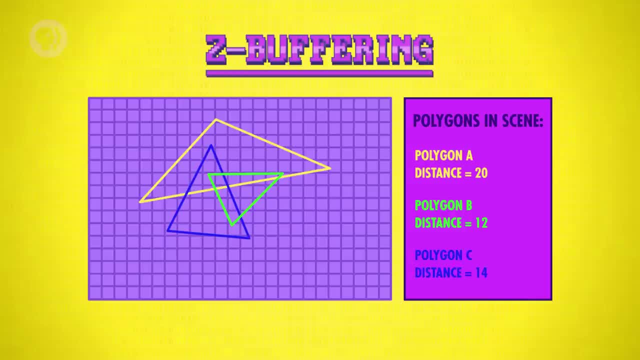 scene. It does this by maintaining a Z-buffer, which is just a matrix of values that sits in memory. At first, every pixel is initialised to infinity. Then Z-buffering starts with the first polygon in its list. In this case it's A. It follows: 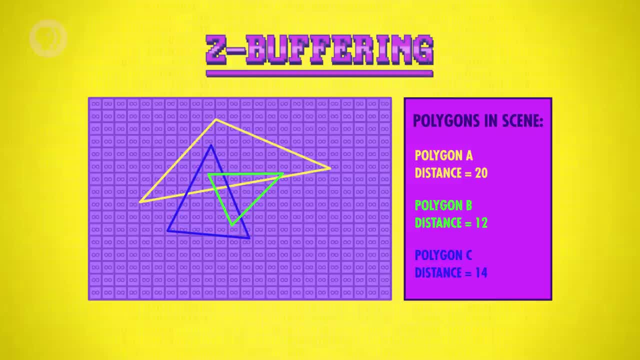 the same logic as the scanline algorithm, but instead of colouring in pixels it checks the distance of the polygon versus what's recorded in its Z-buffer. It records the lower of the two values For our polygon A, with a distance of 20, it wins. 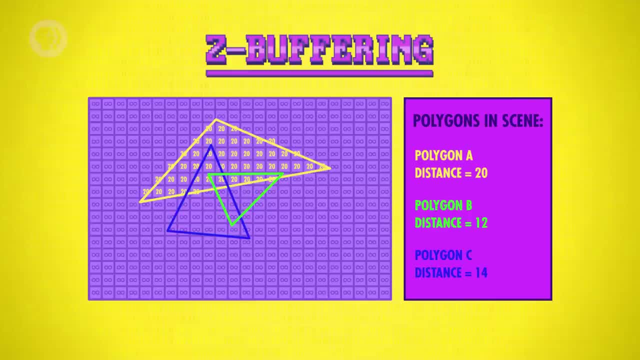 against infinity. every time, No, no, It's over, No, not over polygon in its list, and the same thing happens Now because we didn't sort the polygons. it's not always the case that later polygons overwrite high values. 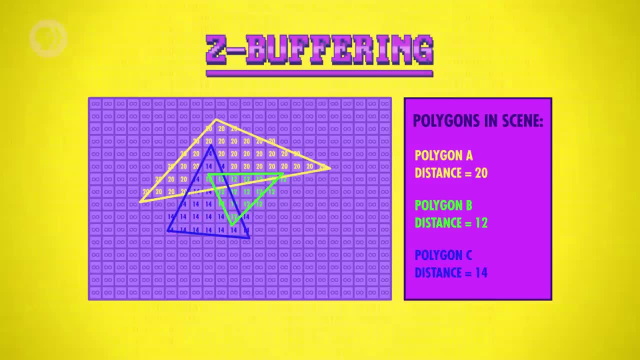 In the case of polygon C, only some of the values in the Z-buffer get new minimum distances. This completed Z-buffer is used in conjunction with a fancier version of scanline rendering that not only tests for line intersection but also does a lookup to see if that pixel 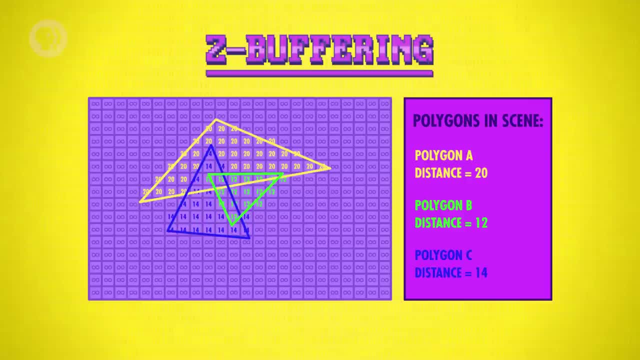 will even be visible in the final scene. If it's not, the algorithm skips it and moves on. An interesting problem arises when two polygons have the same distance, Like if polygon A and B are both at a distance of 20, which one do you draw on top? 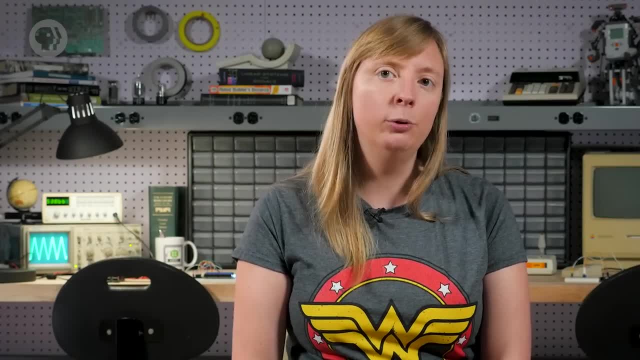 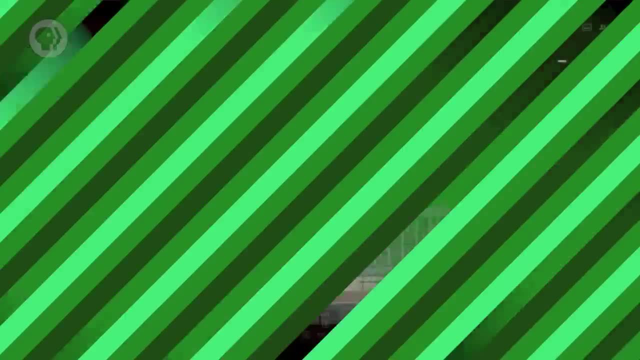 Polygons are constantly being shuffled around in memory and changing their access order Plus rounding. errors are inherent in floating-point computations, so which one gets drawn on top is often unpredictable. The result is a flickering effect called Z-fighting, which, if you've played 3D games, you've 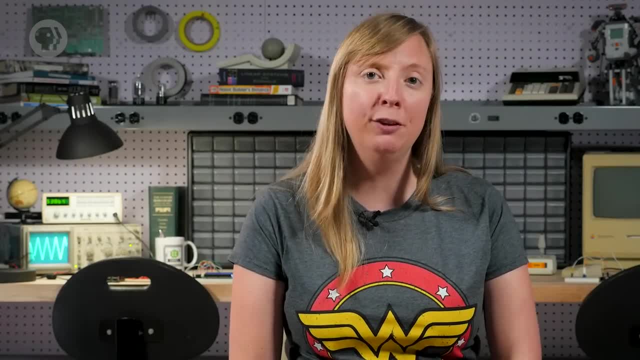 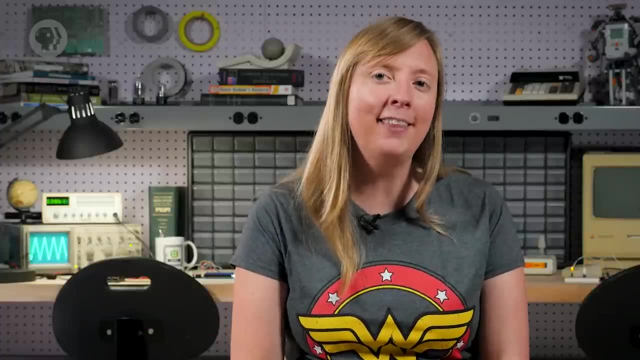 no doubt encountered. Speaking of glitches, another common optimization in 3D graphics is called backface culling. If you think about it, a triangle has two sides, a front and a back, With something like the head of an avatar or the ground in a game. you should only ever. 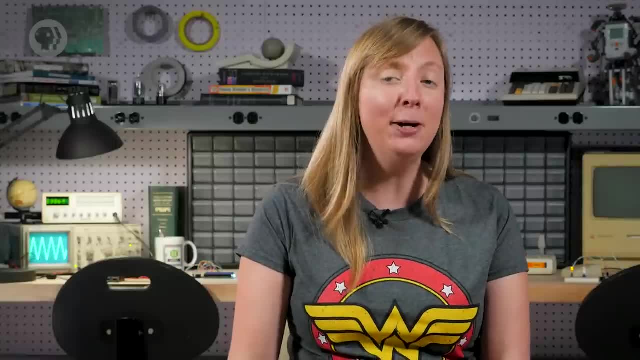 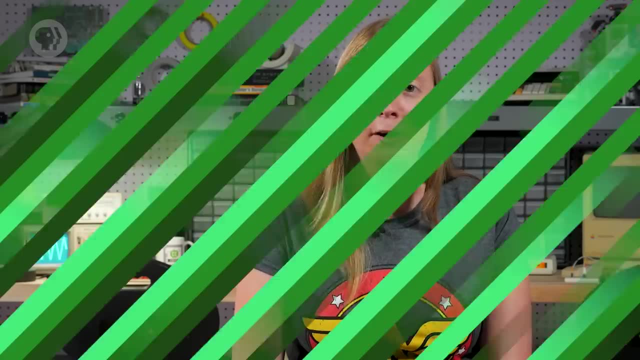 see one side – the side facing outwards. So, to save processing time, the back side of polygons are often ignored in the rendering pipeline, which cuts the number of polygon faces to consider in half. This is great, except when there's a bug that lets you get inside of those objects. 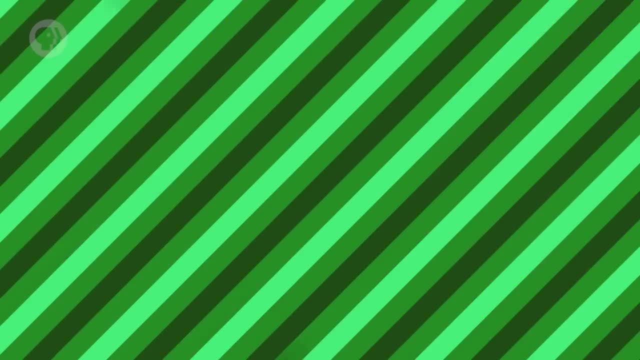 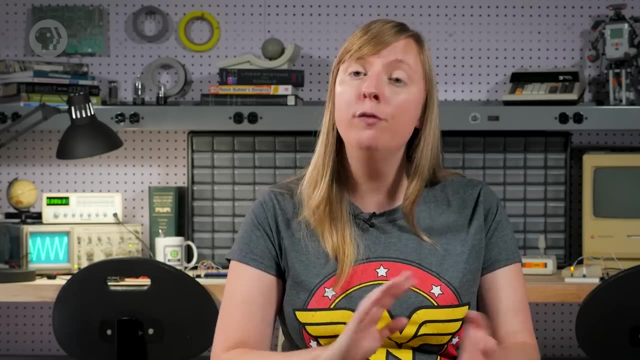 and look outwards, Then the avatar head or ground becomes invisible. Moving on, We need to talk about lighting, Also known as shading, Because if it's a 3D scene, the lighting should vary over the surface of objects. Let's go back to our teapot mesh. 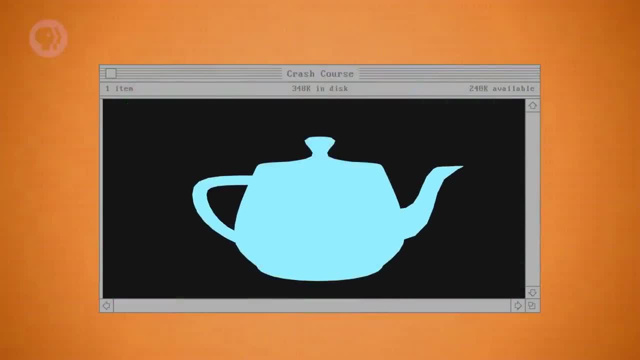 With scanline rendering coloring in all the polygons. our teapot looks like this: Not very 3D, So let's add some lighting to enhance the realism. As an example, we'll pick three polygons from different parts of our teapot. 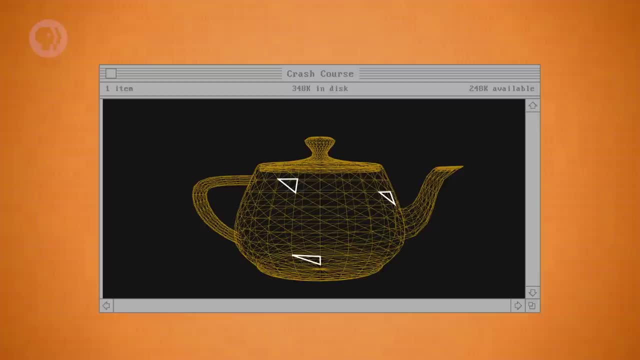 Unlike our previous examples, we're now going to consider how these polygons are oriented in 3D space. They're no longer parallel to the screen, but rather tilted in different 3D directions. The direction they face is called the surface, And we can visualize that direction with a little 3D arrow that's perpendicular to 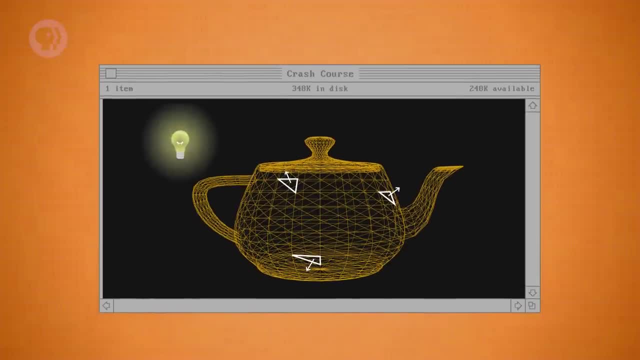 the polygon's surface. Now let's add a light source. Each polygon is going to be illuminated a different amount. Some will appear brighter because their angle causes more light to be reflected towards the viewer. For example, the bottommost polygon is tilted downwards away from the light source, which 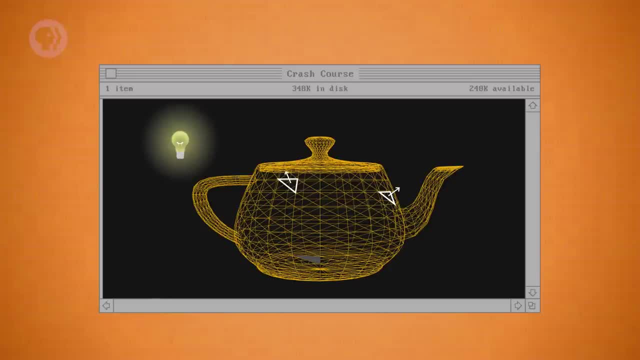 means it's going to be dark. In a similar way, the rightmost polygon is slightly facing away from the light, so it will be partially illuminated. And finally, there's the upper left polygon. Its angle means that it will reflect. It will reflect light from the light source towards our view, so it will appear bright. 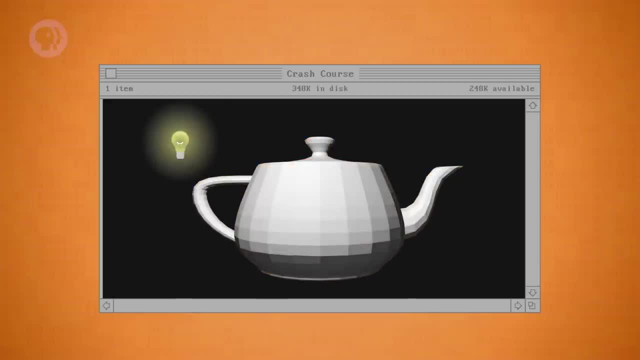 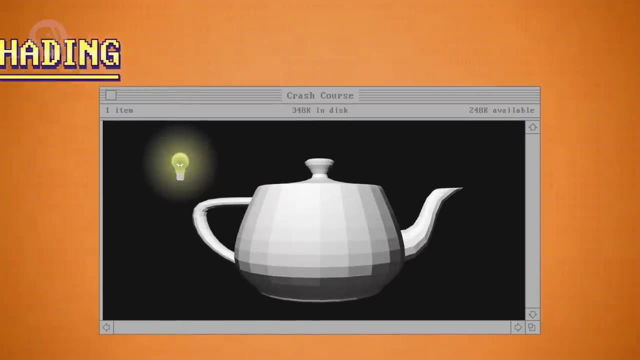 If we do this for every polygon, our teapot looks like this, which is much more realistic. This approach is called flat shading and it's the most basic lighting algorithm. Unfortunately, it also makes all those polygon boundaries really noticeable and the mesh. 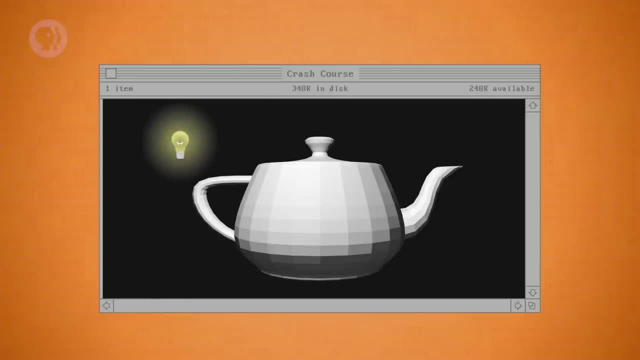 doesn't look smooth. For this reason, more advanced lighting algorithms were developed, such as Gouraud shading and Phong shading. Instead of coloring in polygons, just using one color, they vary the color across the surface in clever ways, Which results in much nicer output. 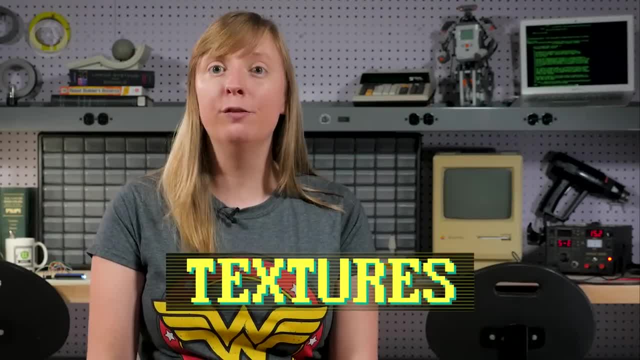 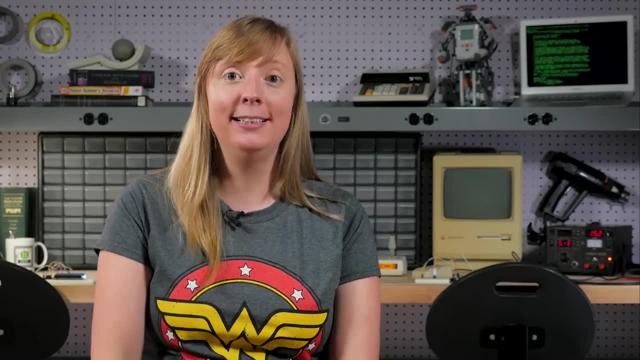 We also need to talk about textures, which, in graphics, refers to the look of a surface rather than its feel, Like with lighting. there are many algorithms with all sorts of fancy effects. The simplest is texture mapping. To visualize this process, let's go back to our single polygon. 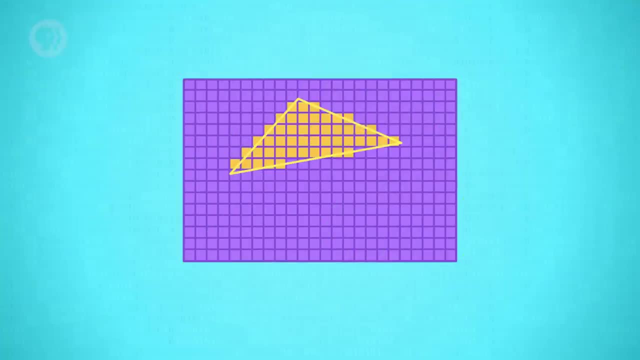 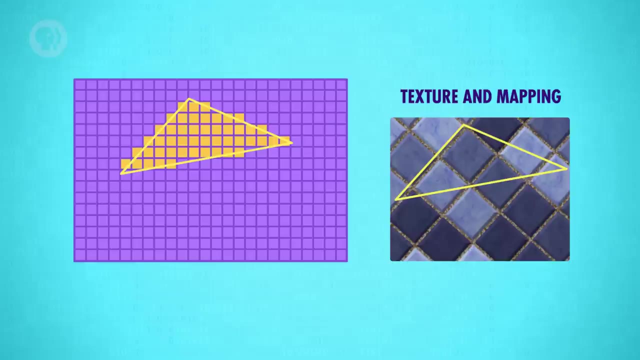 When we're filling this in using scanline rendering, we can look up what color to use at every pixel according to a texture image saved in memory. To do this, we need a mapping between the polygon's coordinates and the texture's coordinates. 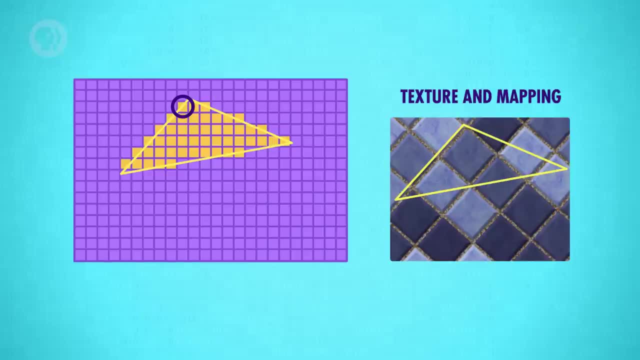 Let's jump to the first pixel that scanline rendering needs to fill in. The texturing algorithm will consult the texture in memory, take the average color from the corresponding region and fill the polygon accordingly. This process repeats for all pixels in the polygon and that's how we get textures. 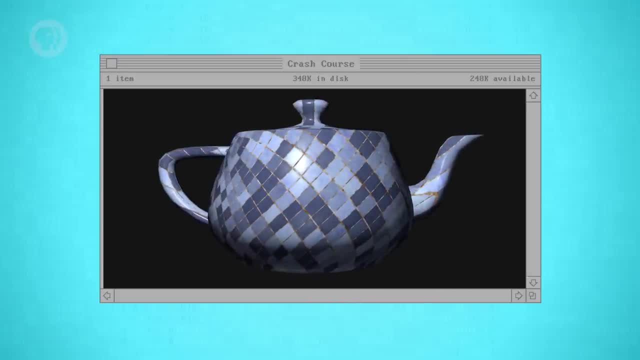 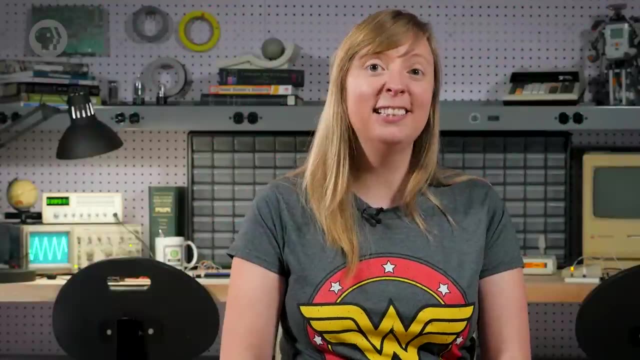 If you combine all the techniques we've talked about this episode, you get a wonderfully funky little teapot, And this teapot can sit in an even bigger scene comprised of millions of polygons. Rendering a scene like this takes a fair amount of computation, but importantly, it's the 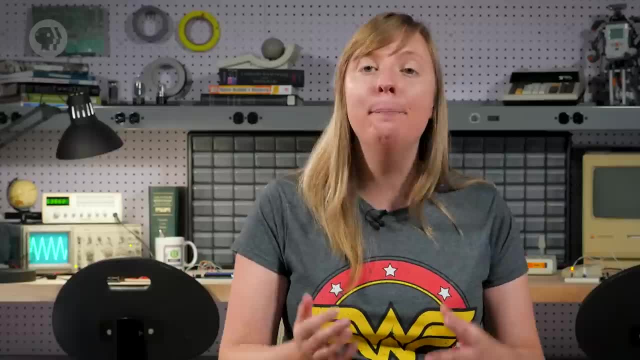 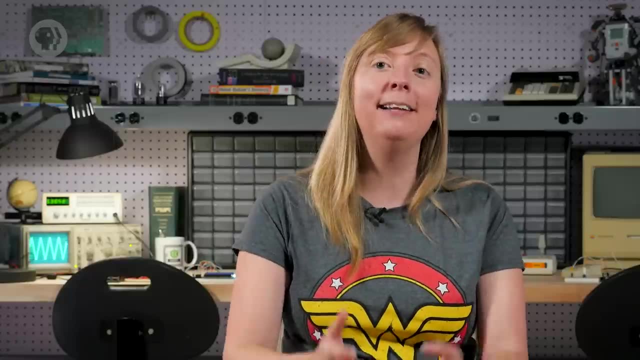 same type of calculations being performed. It's the same type of calculations being performed over and over and over again for many millions of polygons: Scanline, filling, anti-aliasing, lighting and texturing. However, there are a couple of ways to make this much faster. 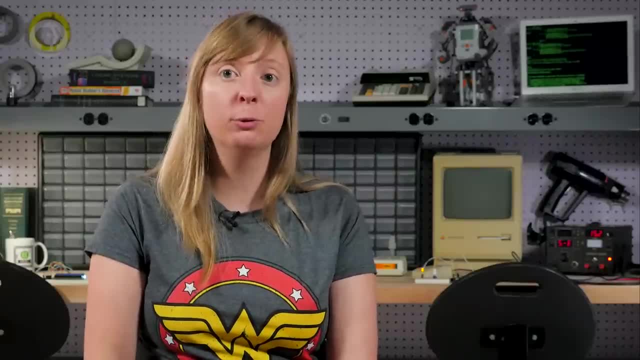 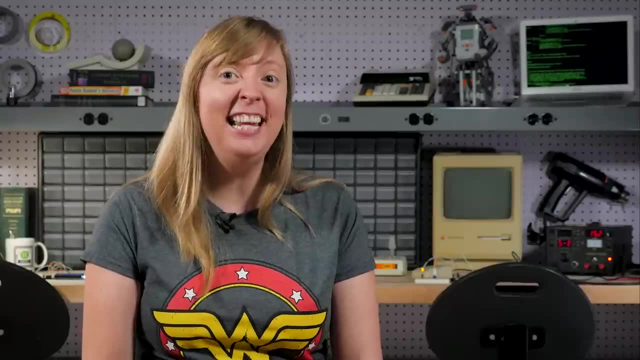 First off, we can speed things up by having special hardware with extra bells and whistles just for these specific types of computations, making them lightning fast. And secondly, we can divide up a 3D scene into many smaller parts and then render all. 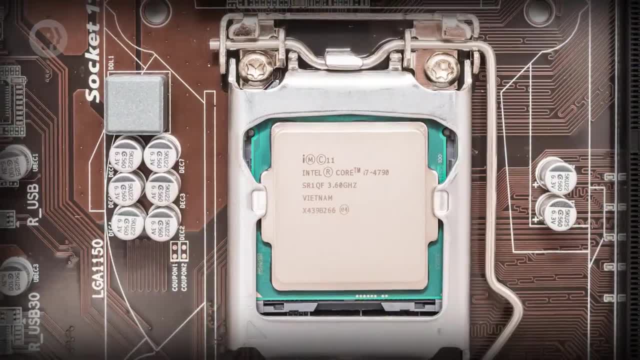 the pieces in parallel rather than sequentially. CPUs aren't designed for this, so they aren't particularly fast. So we can do this with a simple 3D model and then render all the pieces in parallel rather than sequentially. CPUs aren't designed for this, so they aren't particularly fast. 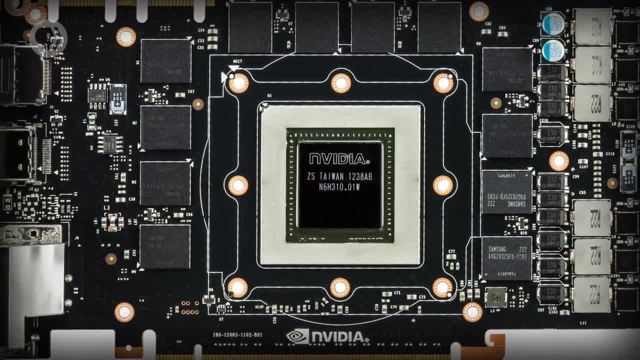 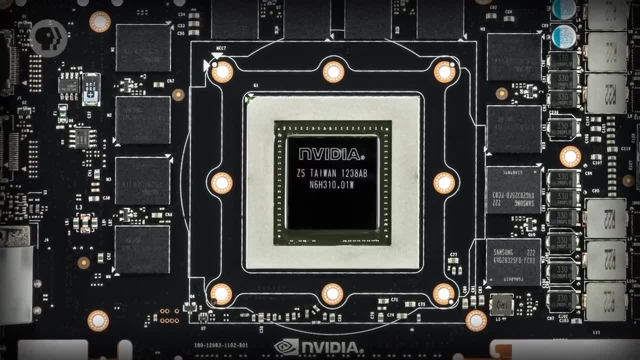 So computer engineers created special processors just for graphics – a GPU or Graphics Processing Unit. These can be found on graphics cards inside of your computer, along with RAM reserved for graphics. This is where all the meshes and textures live, allowing them to be accessed super-fast. 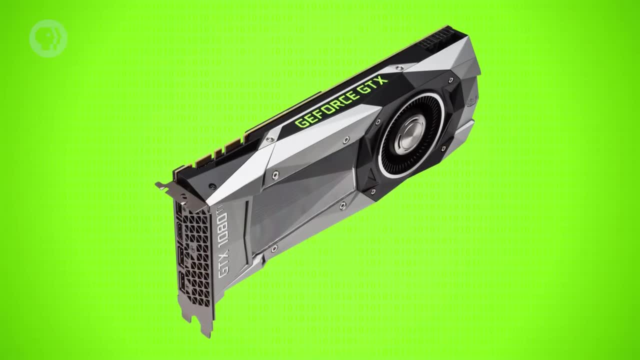 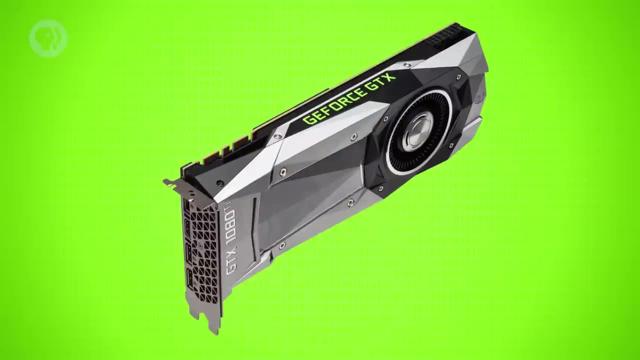 by many different cores of the GPU all at once. A modern graphics card like a GeForce GTX 1080 Ti contains 3,584 processing cores, offering massive parallelization. It can process hundreds of millions of pixels. It can process hundreds of millions of polygons every second.